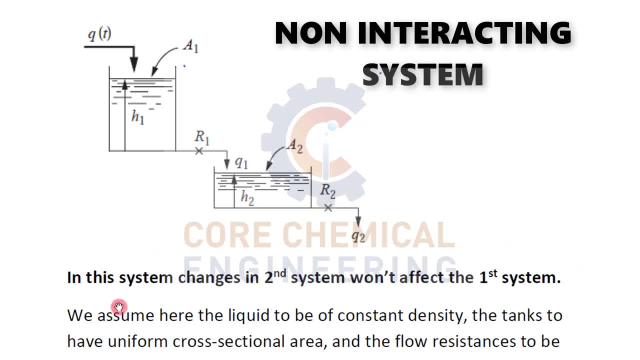 So just remember this: The highlighted, black, highlighted point In this system, What changes in second system won't affect the first system Because you can see it is at a high at this height and after that it is coming to the tank 2 at the lower height. So whenever we are going to change the output in the second system, it won't affect the first system. 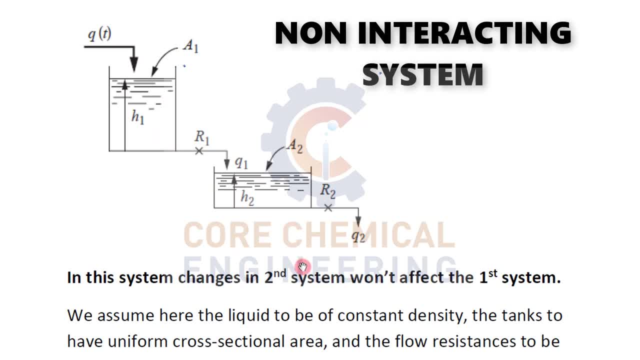 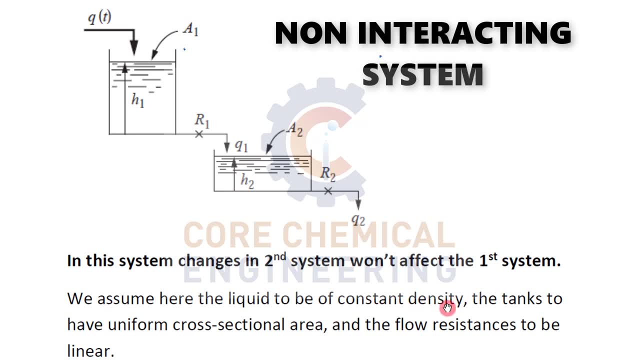 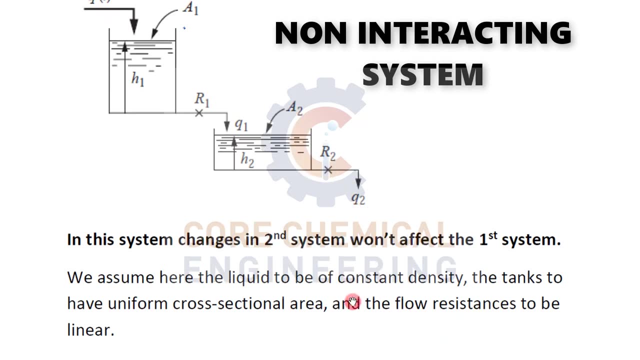 Okay, So that's why we call it as a non-interacting system. Now, in this we assume that here. we assume here the liquid to be of constant density, The tanks to have uniform cross sectional area and the flow resistance to be linear. Okay, And the flow resistance to be linear. 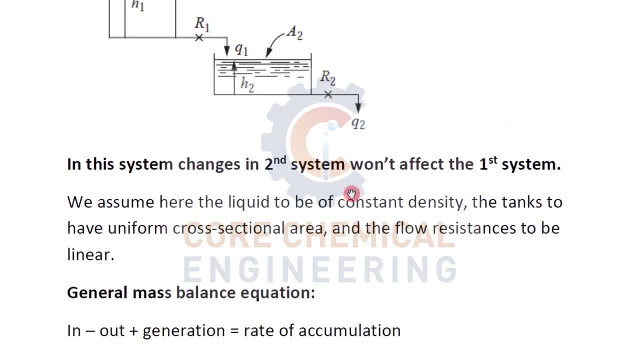 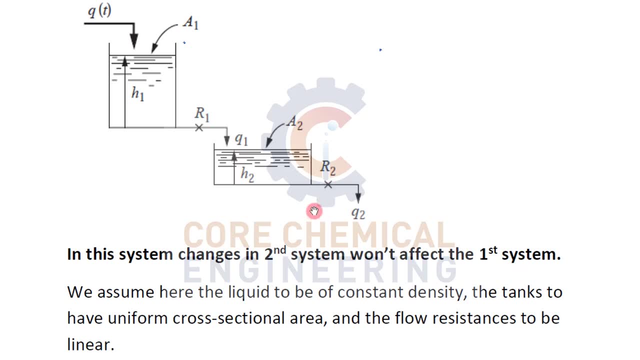 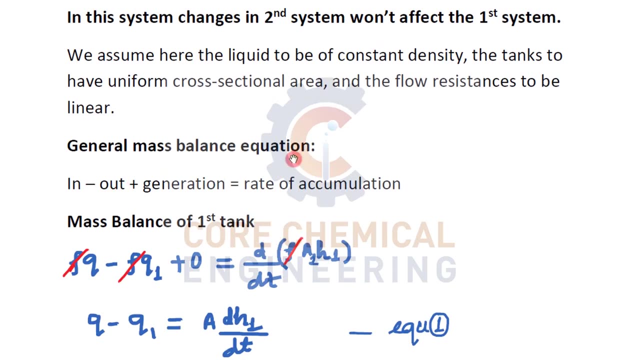 Now How we will get the. you know so how it will get the overall transfer, transfer on first, this kind of non-interacting system. So let the derived that I have this one-by-one. So, as we know, There's the general mass-balance equation by general mass-balance equation in mode. 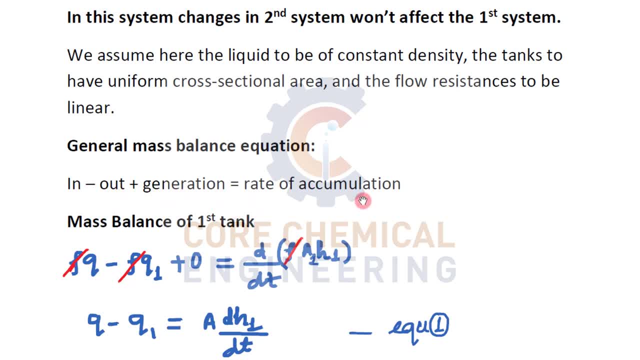 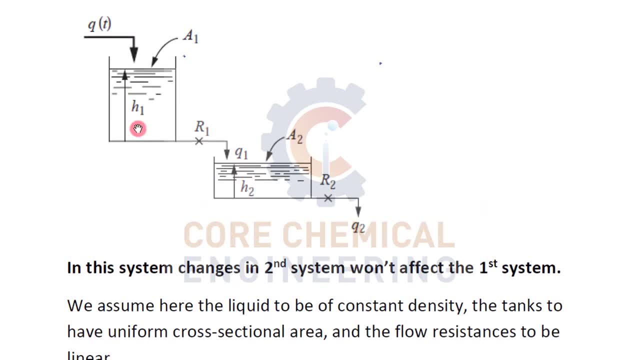 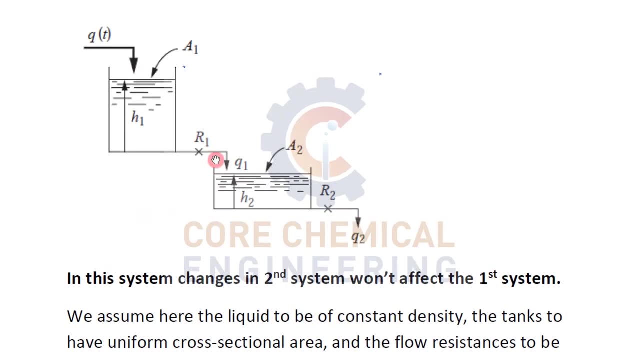 Rate of in minus rate of out of out plus rate of generation is equal to rate of accumulation. so let's do first of all mass balance of first time. so if we are going to do the mass balance of first time, then inlet minus outlet: inlet is Q of T, outlet is Q 1 T. okay so, and generation? because there there is no generation. 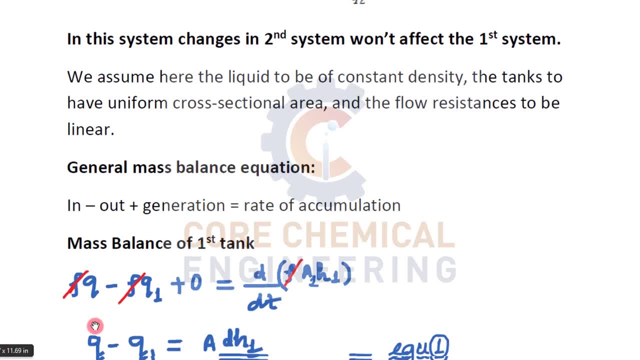 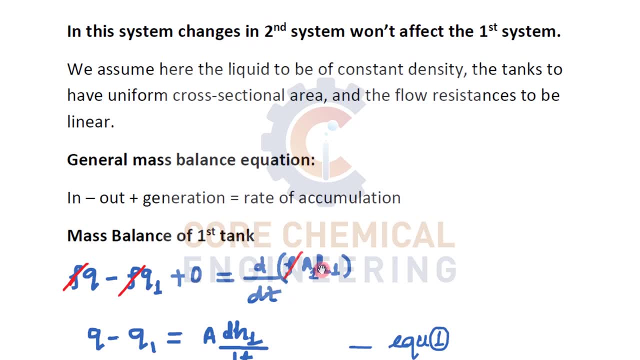 though that can be put at a 0. the row is your, Q is your inlet flow rate and row is your density. row into Q minus row into Q, 1 plus 0 is equal to d y DT. so row into a 1, into H, 1 even is your cross. 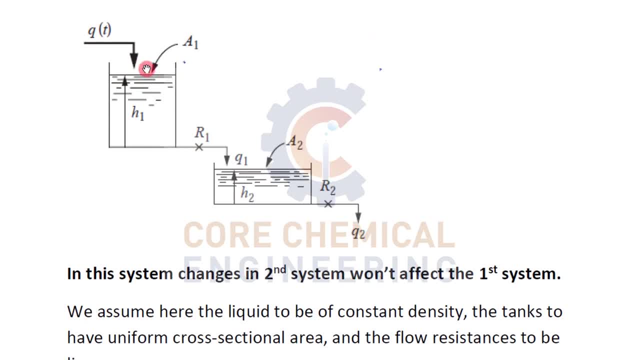 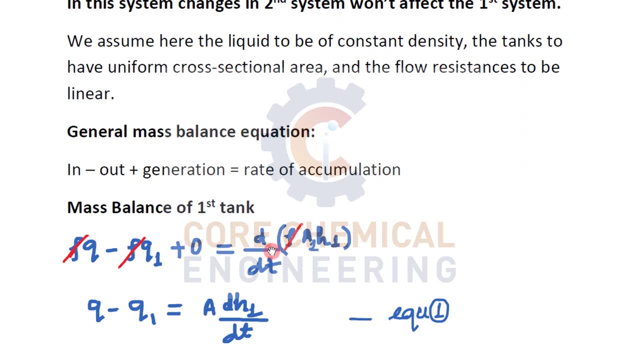 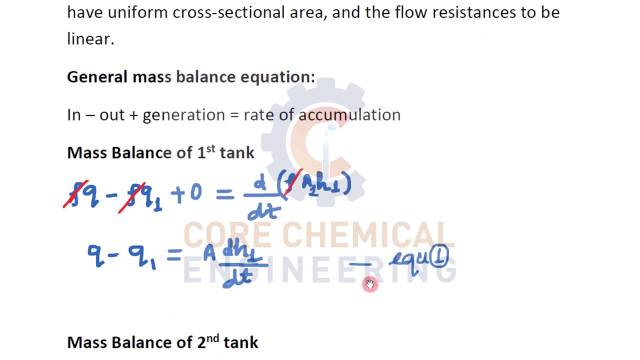 section, area height. so we will get this total cross section. here you have this total cross section, a total volume of the tank, okay, even into H 1. now we can, because density is constant. we can cancel it. we will get the ogran Wij pasteur a Anh and by 13. so we got this one equation now. 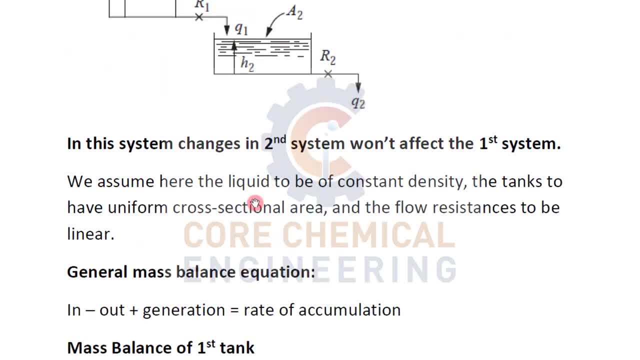 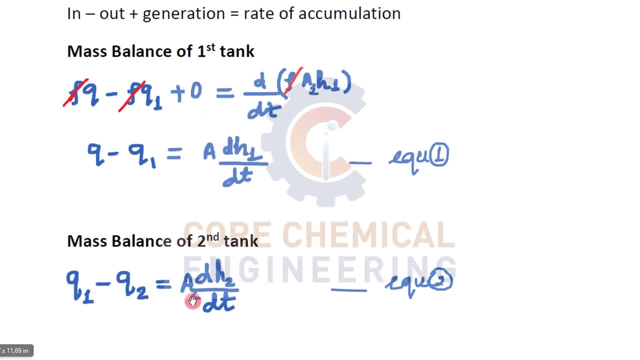 similarly we can do the mass balance for the second time right for the second dig stack. so we get this one equation now. similarly we can do the mass balance for the second time right for the second tank. q1 is the inlet, q2 is the outlet. so q1 minus q2, equal to a2 into dh2 by dt. right here we have. 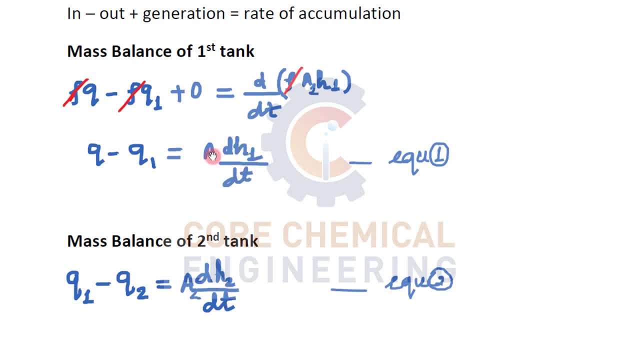 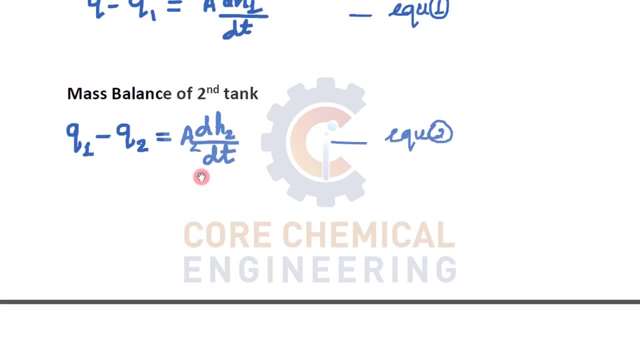 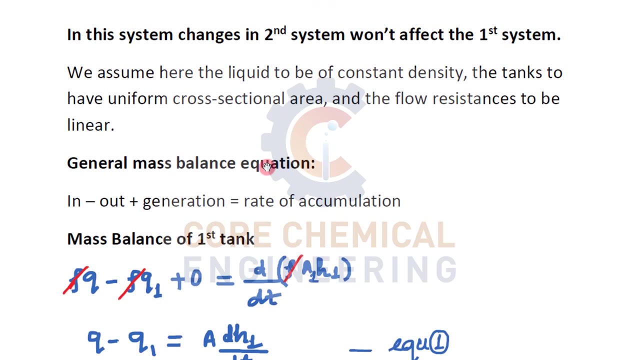 gotten dh1 by dt. here we will get dh2 by dt. this is a1 cross section. it's not a, this is a1. right now we got for the uh. we got the equation for mass balance of the second tank now, as we know, for i had already told the flow resistance to be linear, so because of that, we'll get. 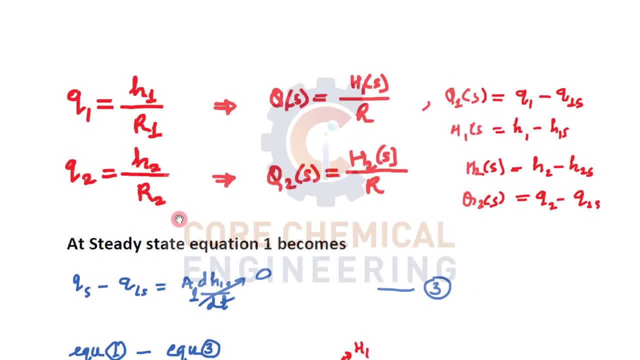 q1 is equal to h1 by r1. okay, q2 is equal to h2 by r2. now your q of n was equal to deviation, like q1 minus q1s. okay, we'll get q1, and if we take the laplace transform of that, we'll get. 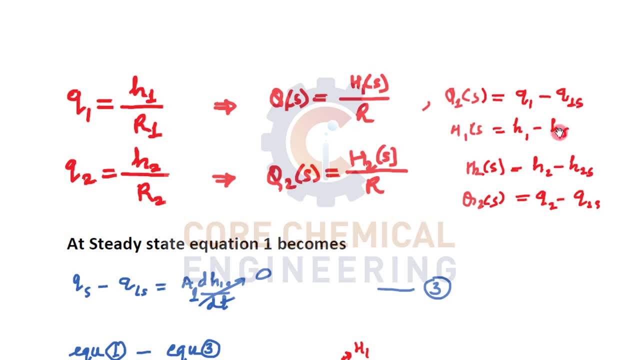 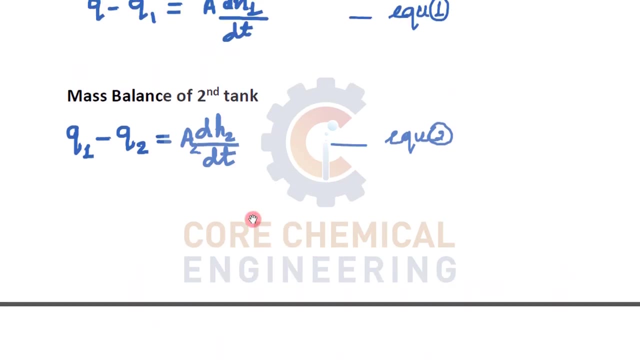 q1 of a. similarly, for that, h1 minus h, inverse h1, this is the steady state value, right. similarly, all those these values will get. so just remember this: q1 is equal to h1s divided by r, and q2 is equal to h2s by r. so, at steady state, first of all, this equation, one right. this is the, for this is not. 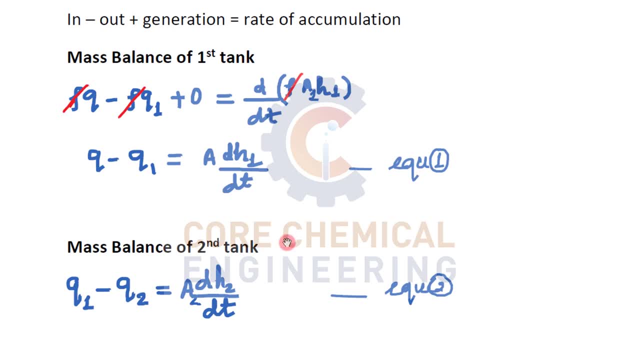 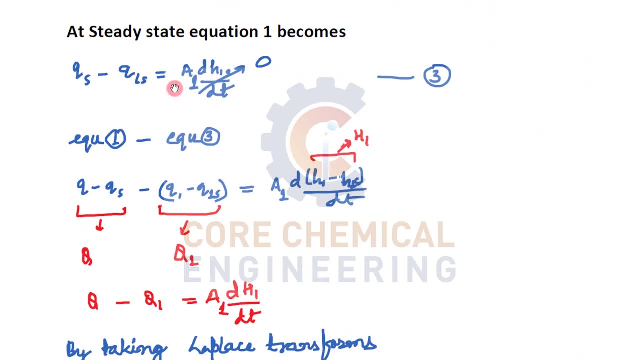 for we had not considered for the steady state condition. now we'll write the equation one same for the steady state condition. so if we write for the steady state condition to, qs minus q1 is equal to a dh1s divided by dt, because height, if it is a steady state, then it is a steady state. 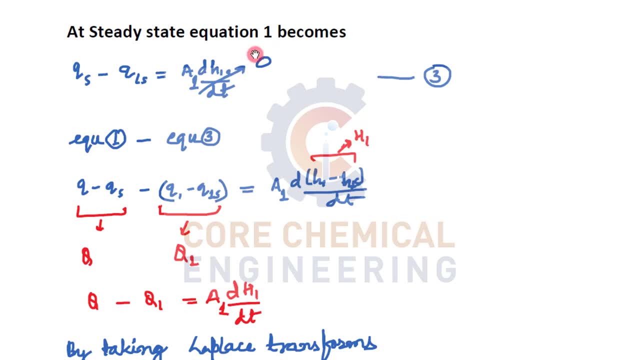 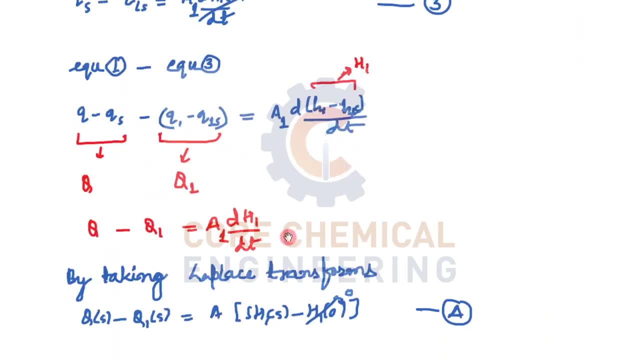 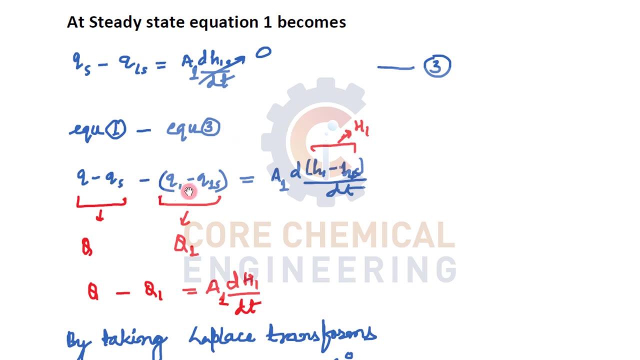 and height won't be changing. so rate of change of height with respect to time would be zero- will get cancelled. so if we subtract equation one minus equation three, so this is your equation one. now we have to subtract the equation three. equation three will get q minus qs, minus of q1 minus q1s. 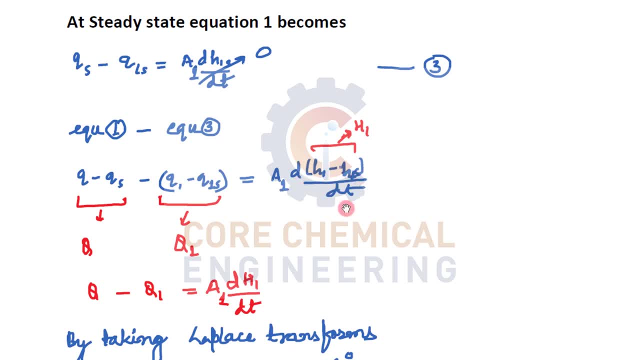 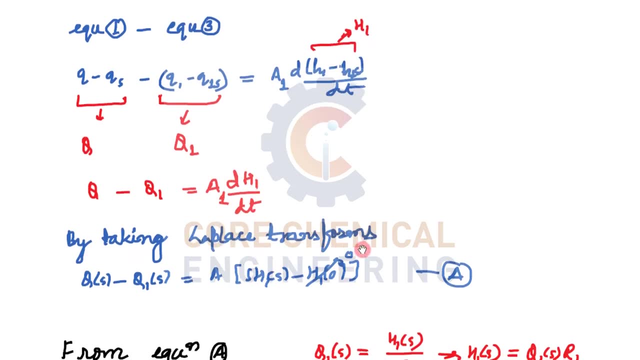 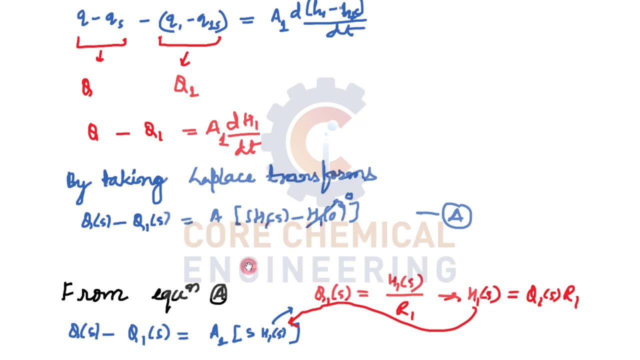 equal to a1 into dh1 minus h1s by dt, right. so for this we'll get value. q minus qn is equal to a1. dh1 by dt, we'll get. qs minus qn is equal to a s of h1s minus hn of zero, so this value would be zero right now. 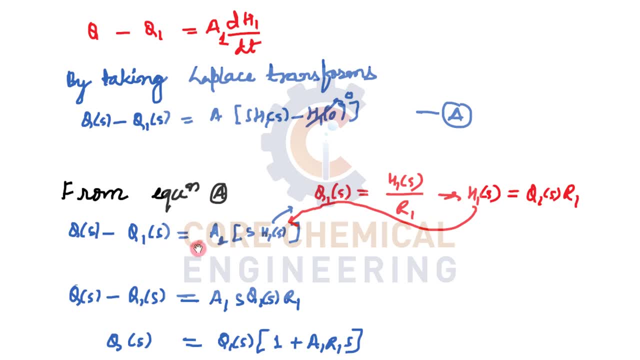 from equation a: okay, qs minus qn is equal to a1s into h h1 of s. we know that h qn is equal to h1s by r1, so we'll get h1s equal to q1 into qn s of r1, so we can put, instead of h1 s we can put: 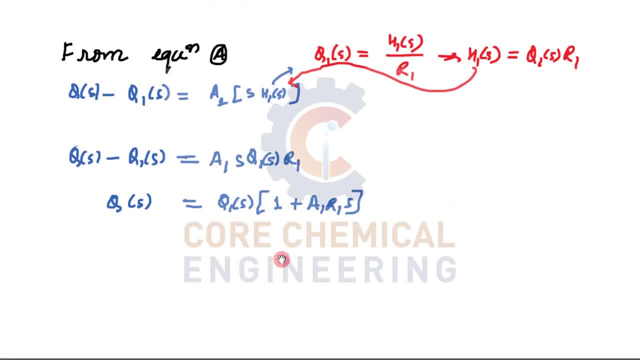 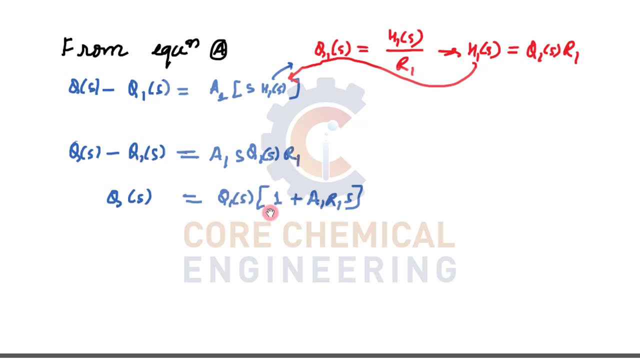 this value qn s into r1 here. after putting that value we'll get qs minus qn is equal to a1s- into qn s, into r1. so take this term this side, and take qn of s in common in the whole. so we'll get qs equal to qn s in bracket into one plus a1, r1 into s. now divide qs divided. 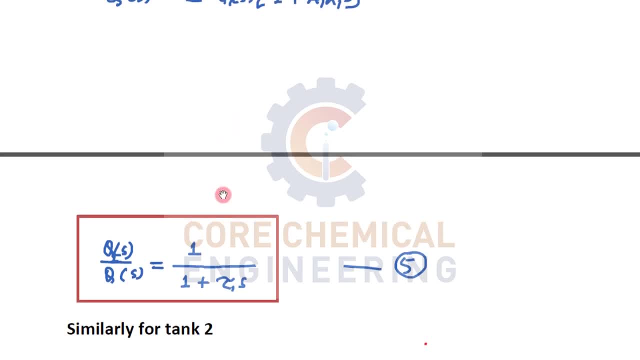 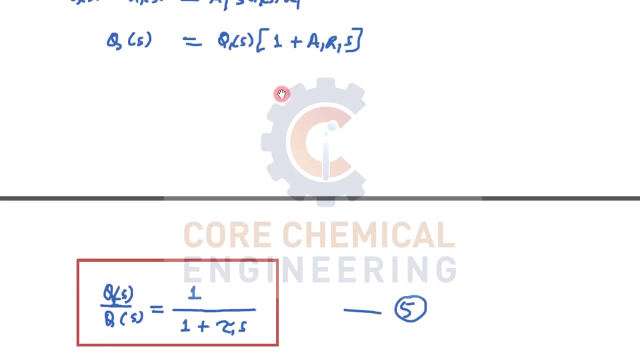 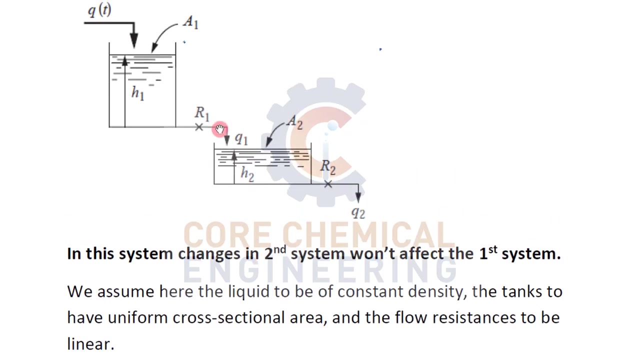 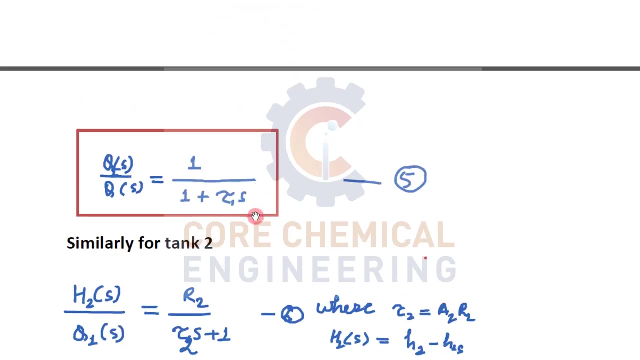 by qn s, divide qn s by qs equal to. so q1 s divided by qs equal to one by one by one plus tau n into s right. so we got the transfer function. so for tank1, qn of s divided by q of s equal to one by- you can see it here- one by tau n plus one. 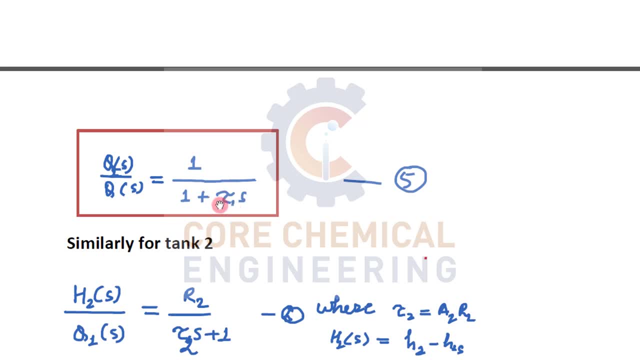 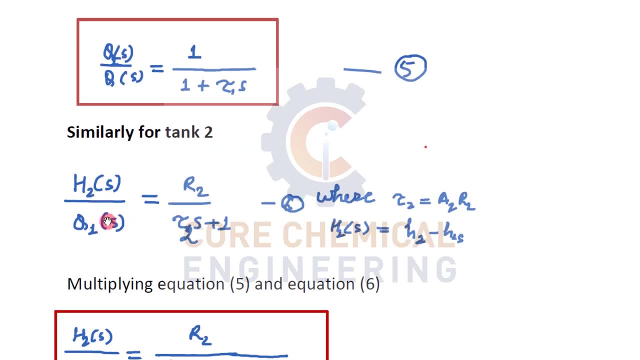 one, divide by one plus tau n s, tau n into s to tau n is your a1 into r1, right for here. similarly for tank two, we'll get h2s by qn is equal to. similarly you can solve for tank two also, we'll get r2. 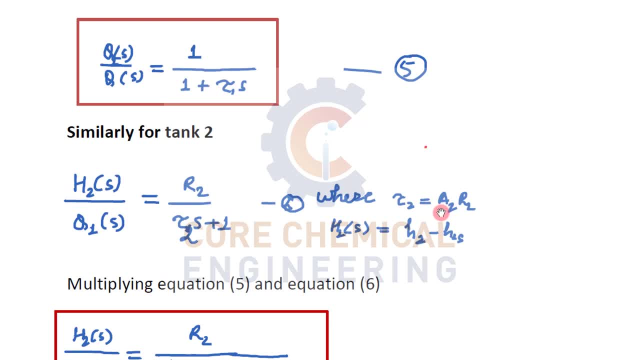 divided by tau 2, s tau 2 into s plus one, where tau 2, your tau 2, would be your a2, into r2, right on h2s here, h2 minus h2s. so if we multiply the equation 4, 5, 5 and the equation 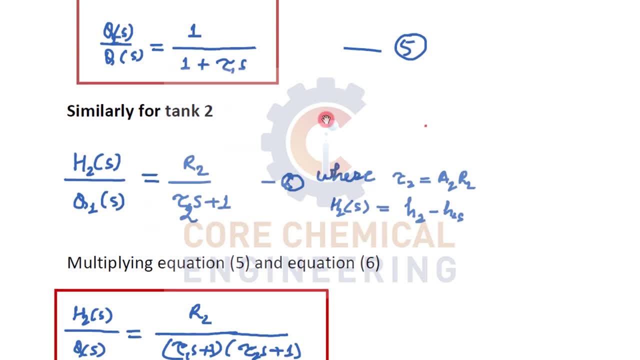 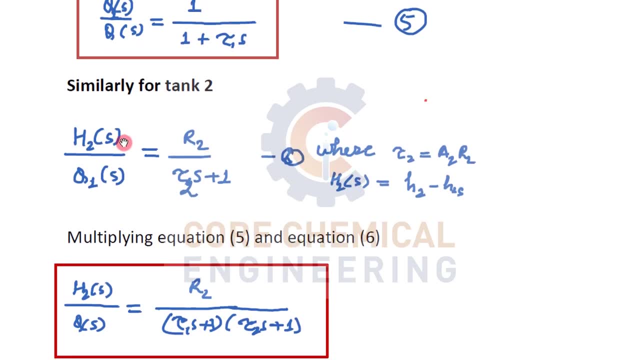 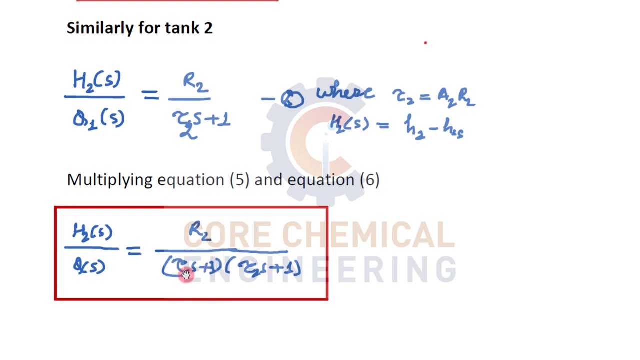 if we multiply the equation this 5 and this equation 6, okay, we'll get this q and s, q and s will get cancelled. then we'll get h2s divided by q of s equal to r2 divided by tau 1s plus 1 in bracket into tau 2s plus 1 bracket close. so from this, okay. 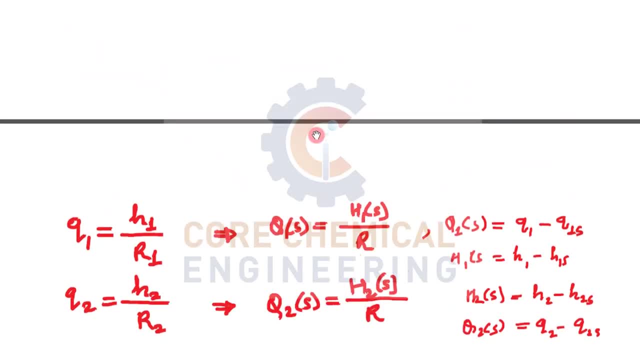 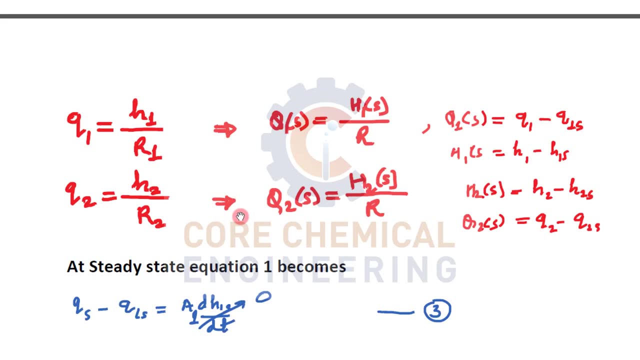 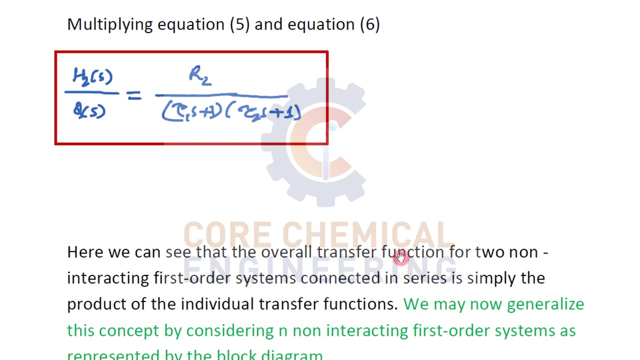 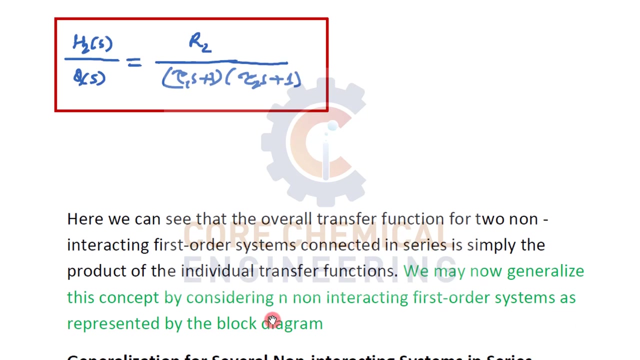 h2. here we have gotten the transfer function. okay, with this h2s. with respect to the q of s, we got this value. so from here we can see that the overall transfer function for two non-interacting first order system connected in series is simply the product of the individual transfer. 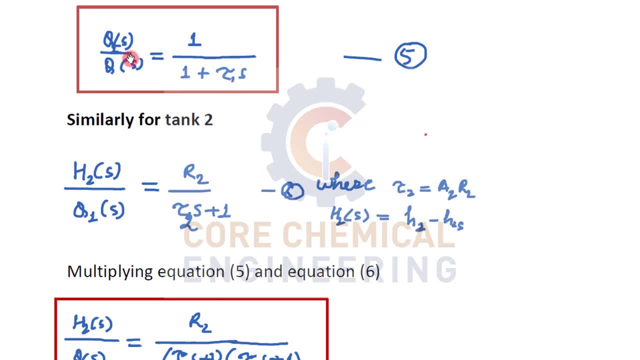 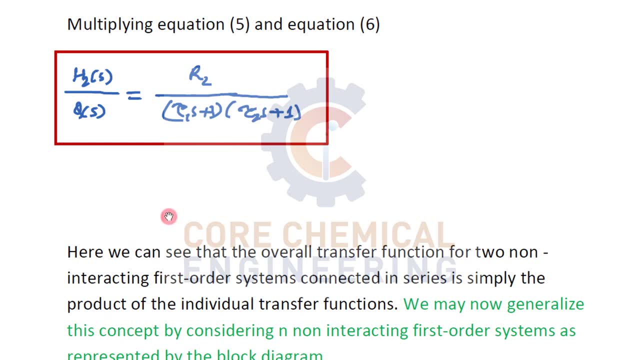 function. simply make a care. is transfer function? is transfer function? go multiply here or I mean it overall transfer function, will be okay. so you have some may generalize. consider we can generalize that that here we can see that the overall transfer, overall transfer function for the two non 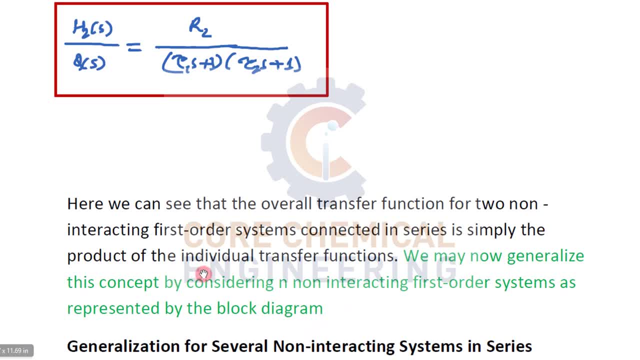 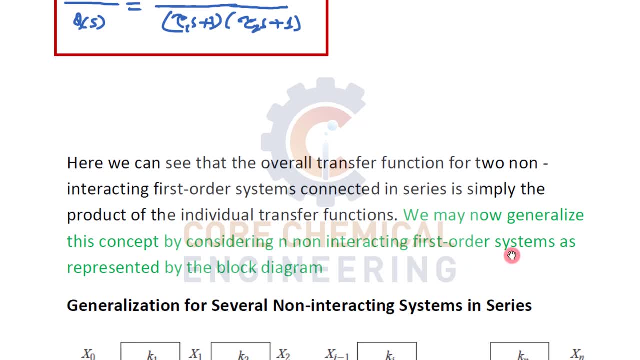 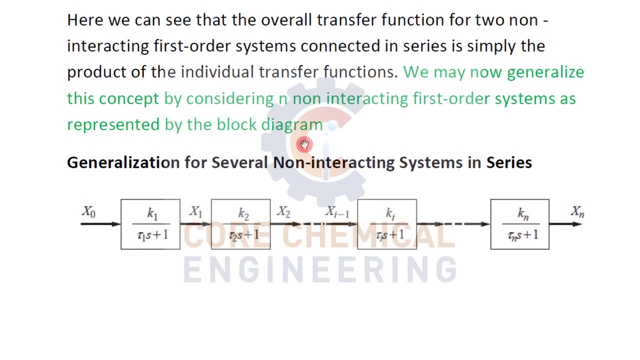 interacting first order system connecting in series is simply the product of the individual transfer functions. so B may now generalize the concept by considering and non-interactive first order system as represented by the block diagram. so suppose that was the for only for two systems. suppose we have similarly n n systems then, and here I had represented 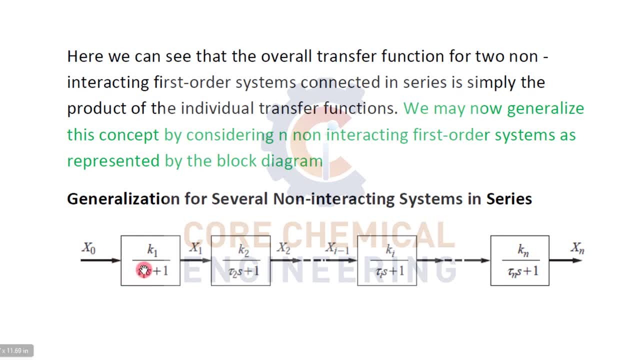 that n system by this block diagram. okay, like given, divided by tau, n s plus 1, output x 1. then K 2 divided by tau, 2 s plus 1, similarly key I divided by tau, I s tau into s plus 1. so these are the 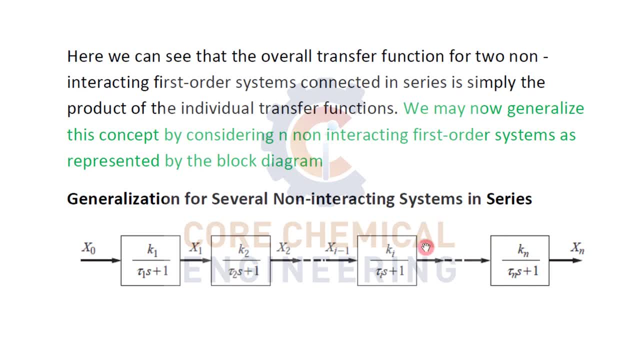 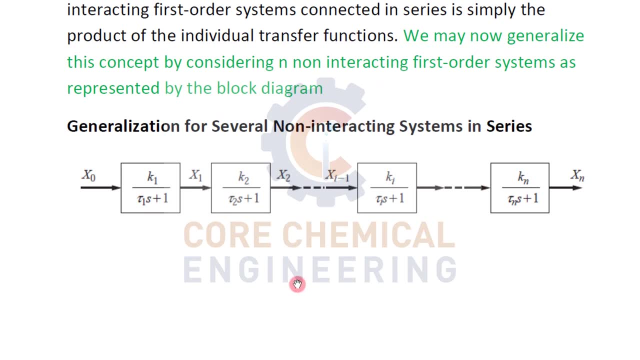 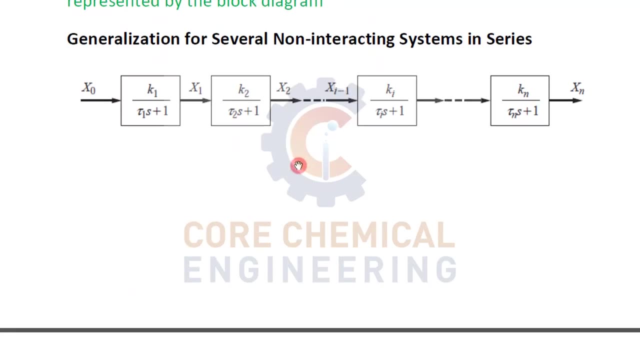 I'm n non-interactive systems. they are connected in series. so how will get so if we generalize that simply, we can multiply the all transfer functions if we want to calculate the overall transfer function of n non-interactive systems in series. so x1 by x naught h. x1 divided by x naught h will. 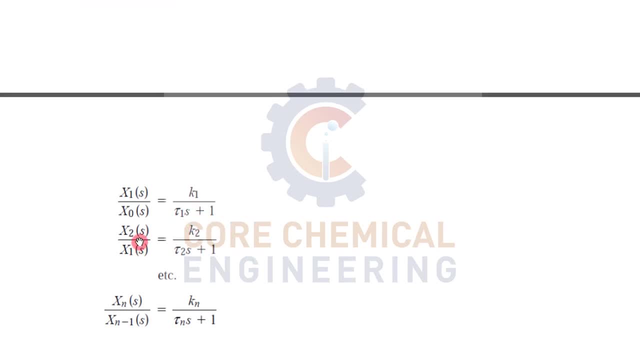 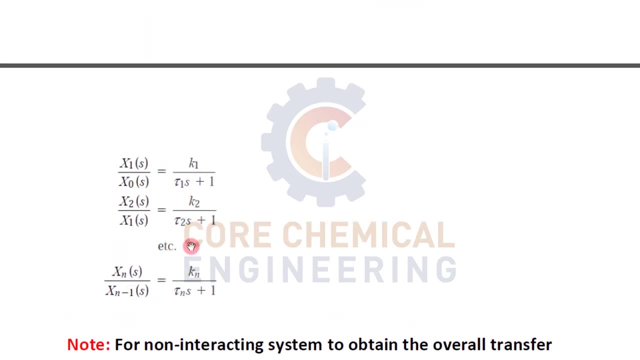 get k1 divided by tau 1 tau n s plus 1, similarly x2 s. x2 s divided by x1 s equal to will get k2 divided by tau 2 s plus 1, etcetera. so similarly, for total value, x1 divided by x n minus 1 is equal. 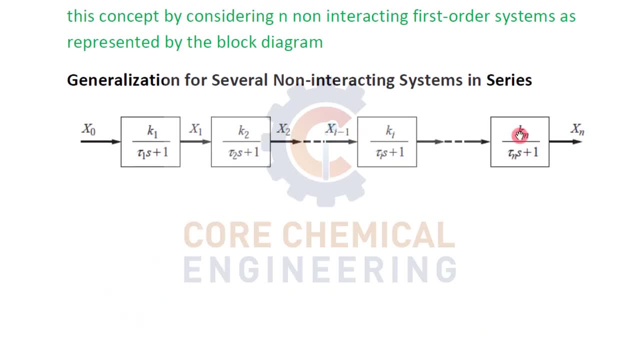 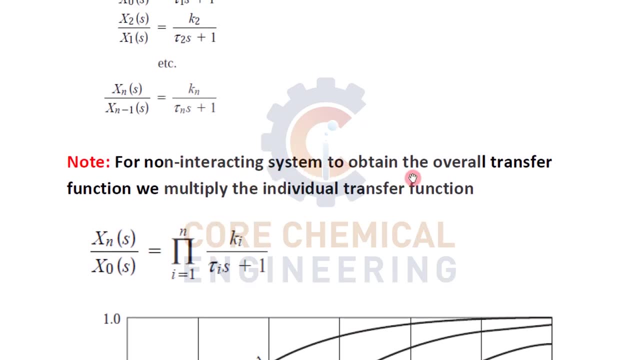 to k 1 divided by tau n s plus 1. okay, this is for with respect to this. now for non-interactive system: to obtain the overall transfer function, we multiply the individual transfer function. so, similarly, this this is what we will get: x n s squared by x naught is equal to: 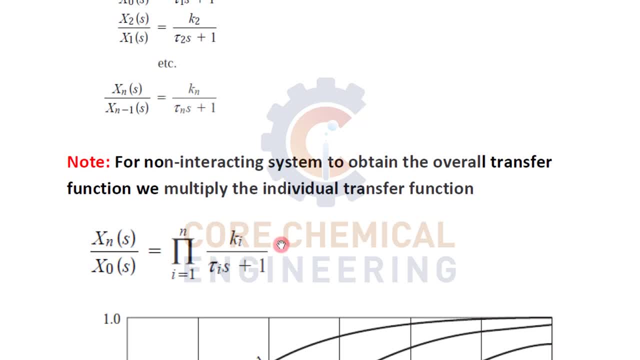 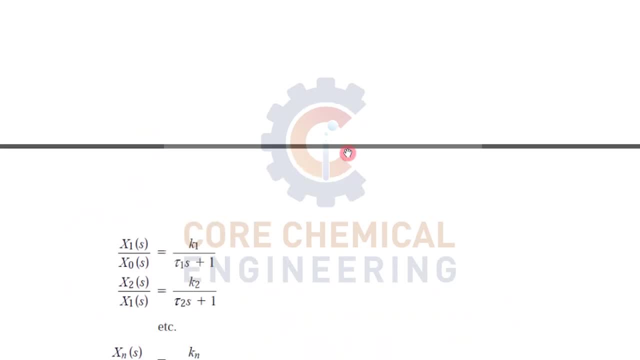 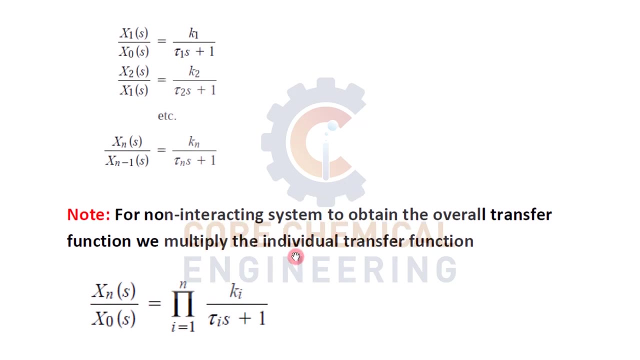 multiplication of from i is equal to 1 to n ki divided by tau i s plus 1. so you must remember this general formula. even you don't need to remember, you just multiply. three systems are given like that. you have to multiply all the three systems right in order to get the overall transfer function for that systems in connected. 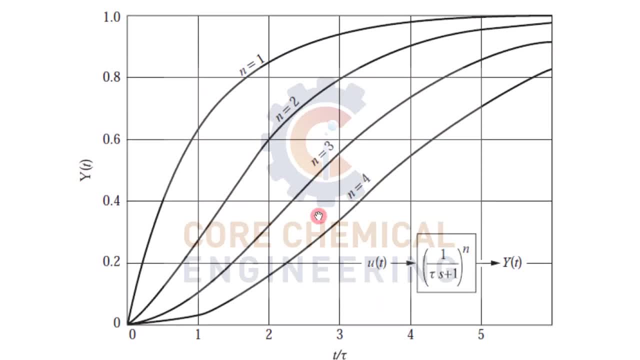 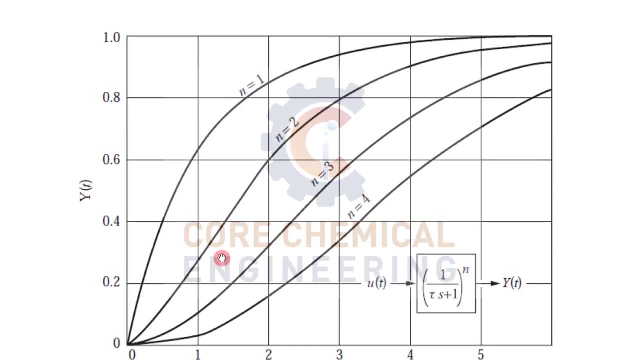 in series, right? so this is the graph represented for for that. this is y by t output. okay, this is t by tau. so for first order, we'll get the graph output graph by like this: for this: if n, two system are connected in series, then we'll get the output like this: if three like this, then four like this: 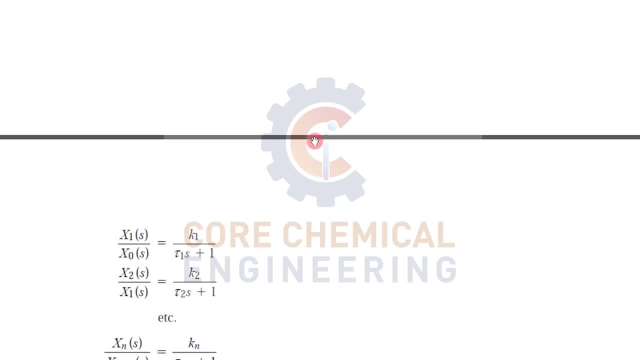 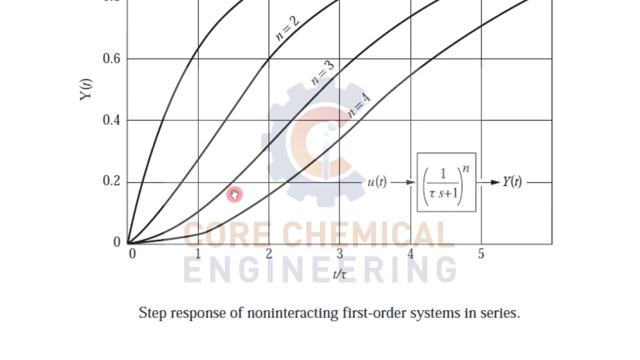 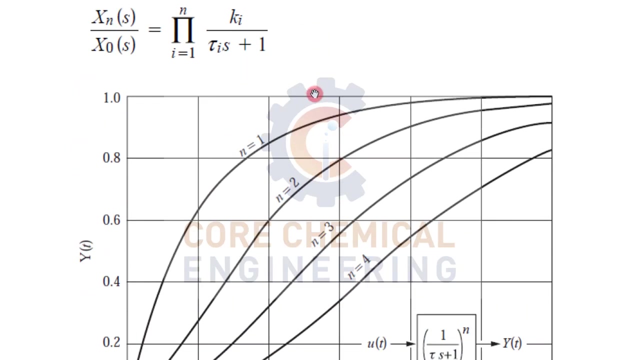 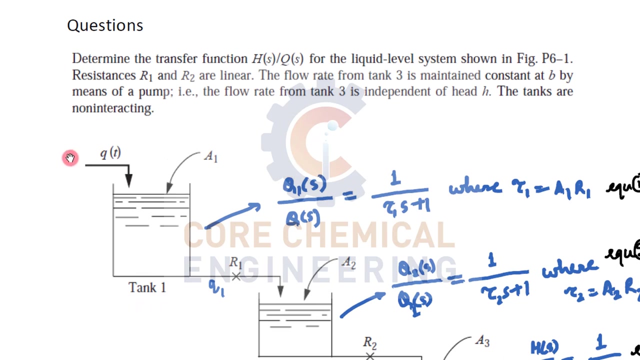 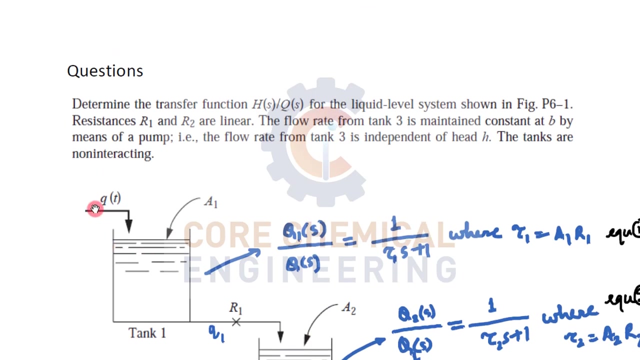 okay, so as we increase the number of tanks, then your output response time will decrease. right, output response time will increase. now, based on, based on the concept of non-interacting system, will solve two numerical problems. okay, so here. one question is written here: determine the transfer function of h of s, h of s divided by q of s for the liquid. 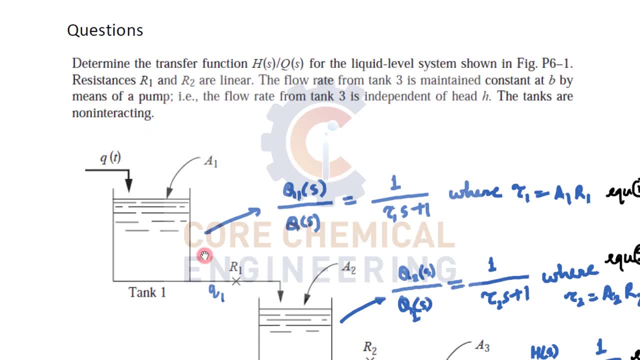 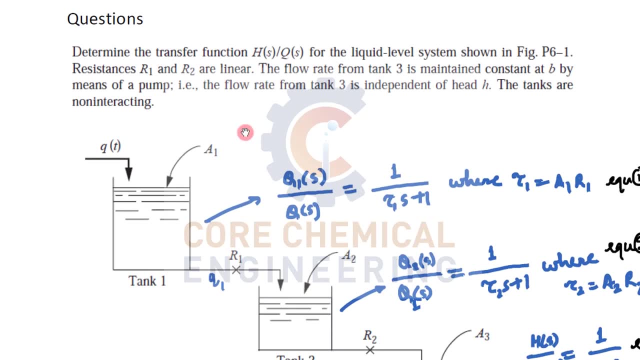 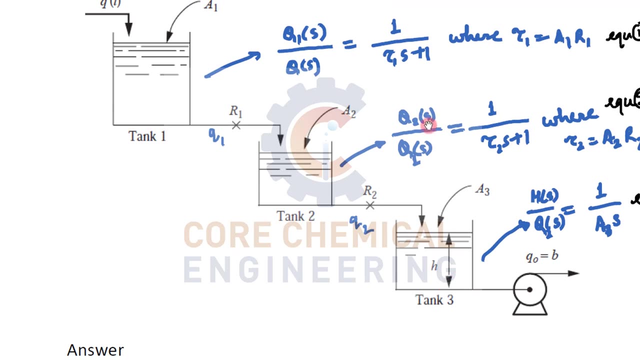 level system shown in figure this. okay, resistance r1 and r2 are linear. the flow rate from the tank 3 is maintained by constant at v. okay, by means of pump the flow rate from the tank 3 is invented of head to flow rate from the pump is independent of head right. the tanks are non-interacting, so 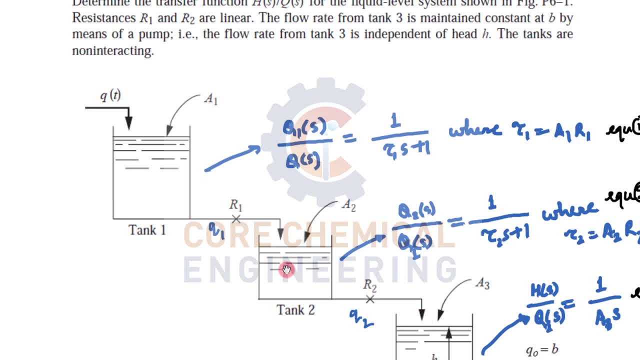 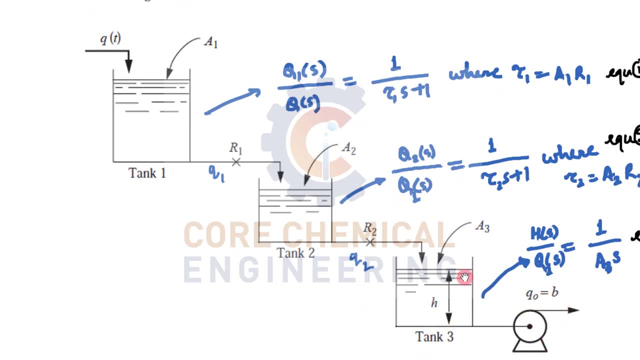 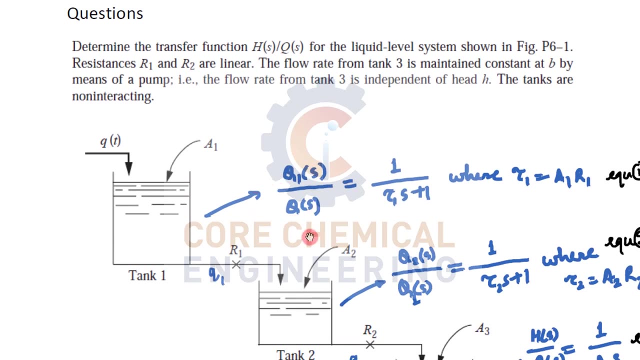 given tanks are non-interactive system. r1, r2, resistance are linear and here flow rate is maintained constant and it is not dependent on height s. so simple, simply, i had already told you, in order to calculate the transfer function of a different tank system are connected in series. okay. 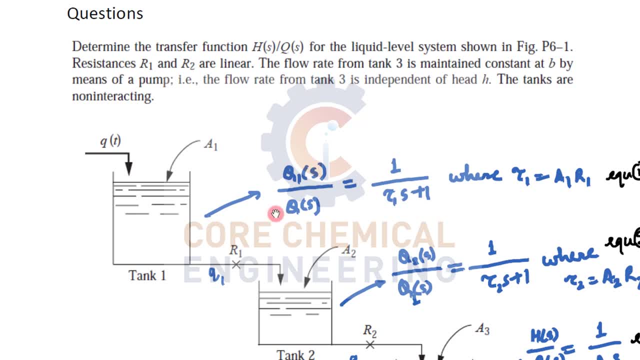 if they are non-interacting, then you have to multiply simply the transfer function of individual systems. so for this you have to write the transfer function. for this time you can derive it. i had already told you that you have to write the transfer function, for this time you can derive. 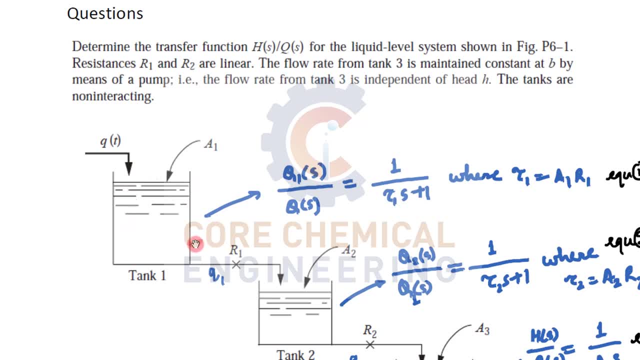 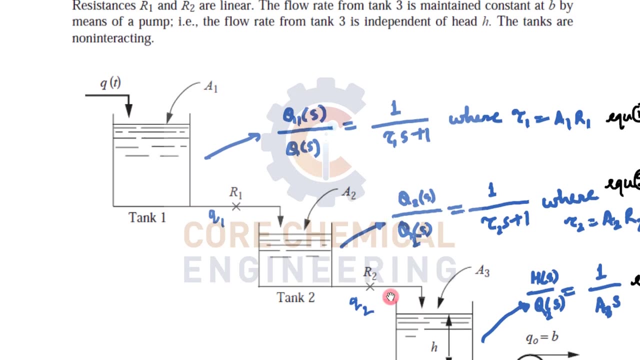 it. i had already told you how to derive. derive the transfer function for individual tanks by doing the mass balance. okay, so q of n s divided by q of s is equal to 1 divided by tau 1 s plus 1, where tau 1 tau 1, tau 1 for this one is a1 into r1. for this system, q 2 s divided by q 1 s is equal. 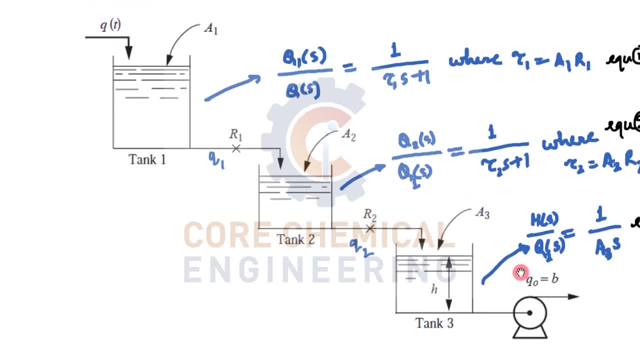 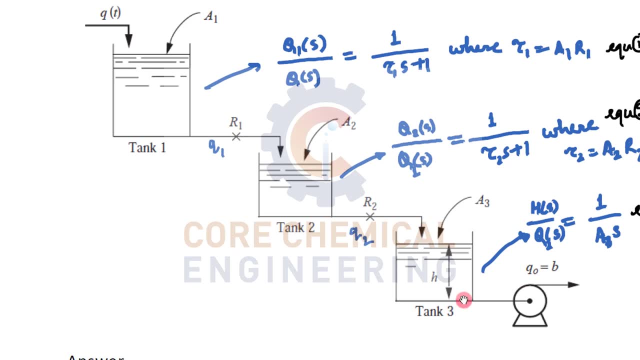 to 1 divided by tau 2, s plus 1. okay, where tau 2 is equal to a2, r2. for this, one hs of divided by q, q1, 2 of s is equal to 1 divided by a3 into s. okay, so what we need to do in order to get the hs divided: 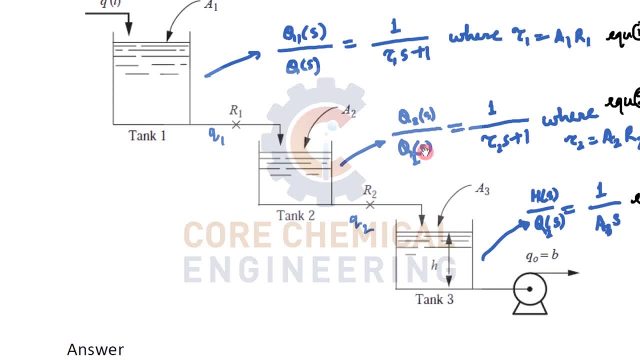 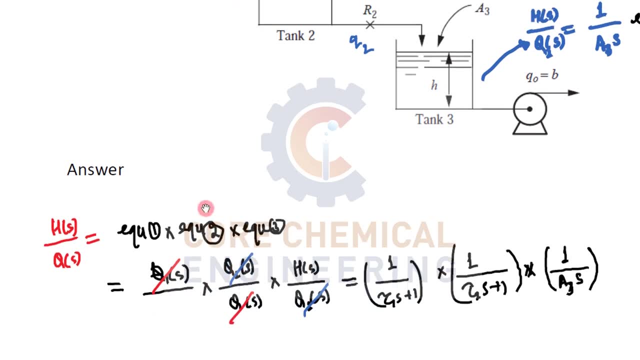 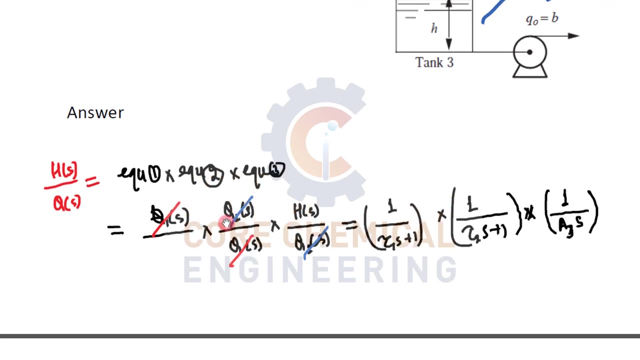 by q of s. multiply equation one, two and three. multiply one, two and three, we'll get hs divided by q2 of this. here q2 of s will come. okay, uh, q1 is divided by q of s. here q of s will come. then here again, q1 is divided by q of s. then here hs divided by q2 of s. all these will get. 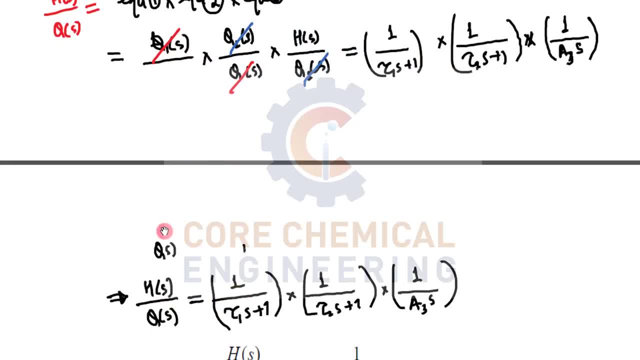 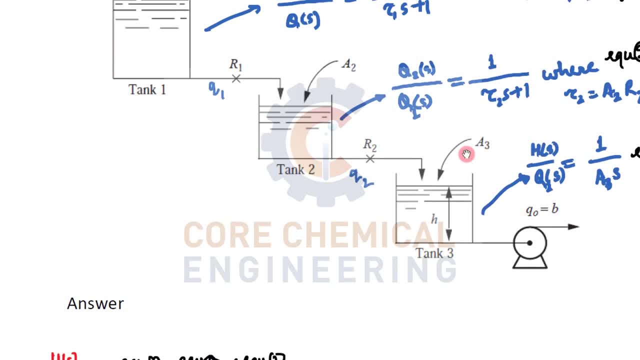 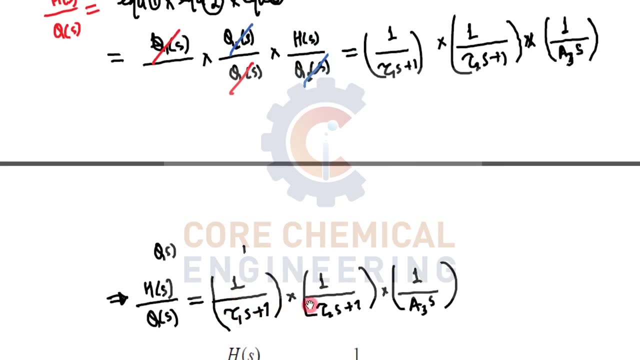 will get cancelled, but we'll. we'll get finally. okay, this q of s came here. instead of that, we'll get h of s divided by q of s equal to now. we have to multiply the individual transfer function 1, 2 and 3, so we'll get this in this form. we'll get 1 divided by tau, 1, tau 1 s plus 1 into 1 divided. 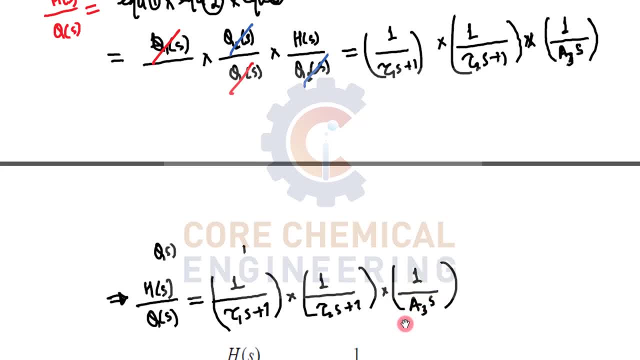 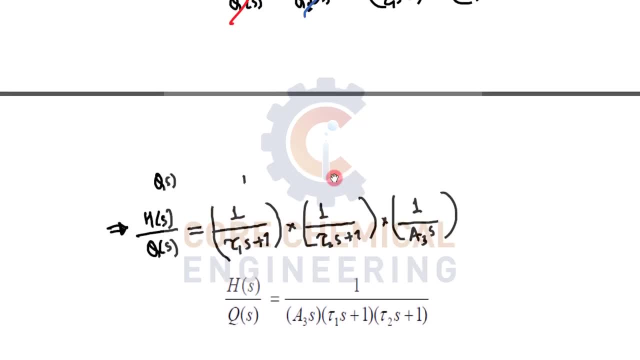 by tau 2 s plus 1 again into in bracket 1 divided by a3 into s. so overall this value will get. so this is how we can easily calculate the- you know- overall transfer function on for non-interacting system. if we know the fundamentals and if we have the clarity. 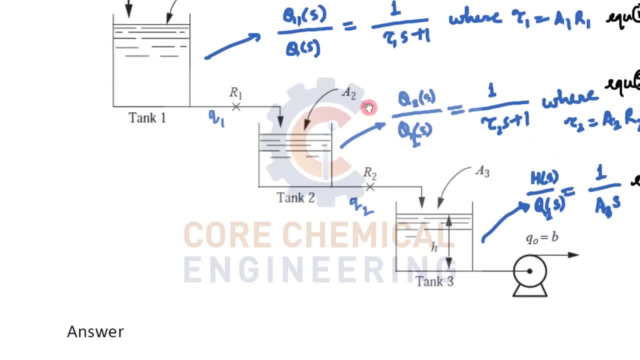 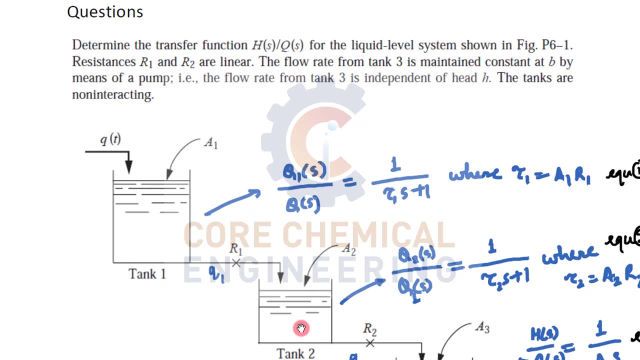 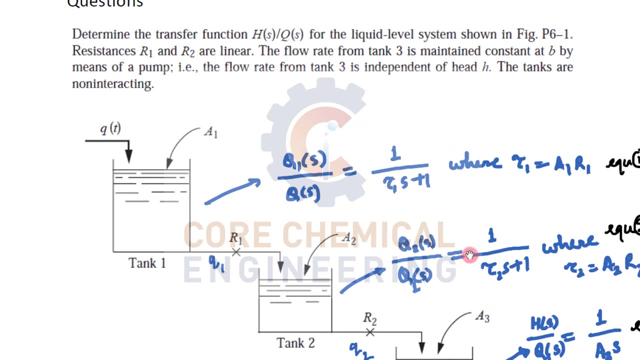 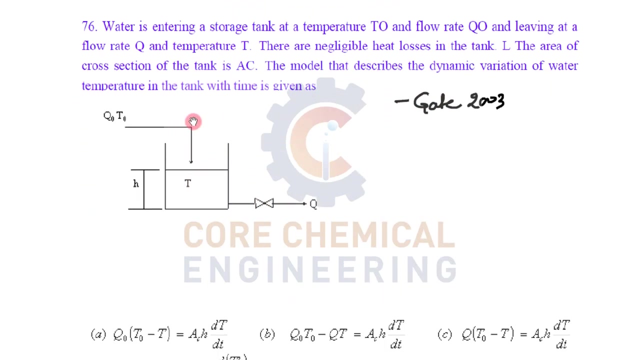 for the concept for non-interacting system. so simply, simply, we have to write the transfer function for individual, individual tanks and then multiply. all okay. now one more question is there? um, that was asked in the gate, exam 2003. water is entering a storage tank at a temperature t naught. 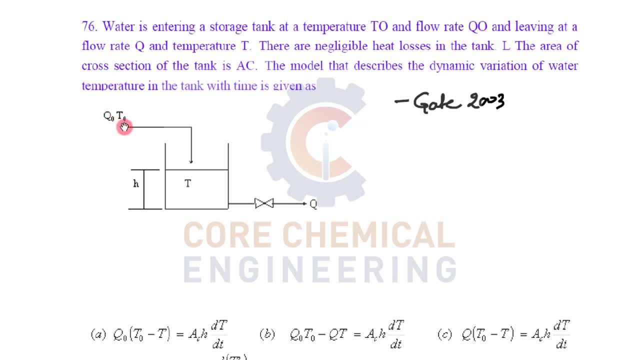 this is not to t naught and the flow rate q naught, okay, q naught and the flow rate is q, not okay. and leaving at a flow rate q, living at a flow rate q and temperature t, so temperature t same as outlet, there are negligible heat losses in the tank. 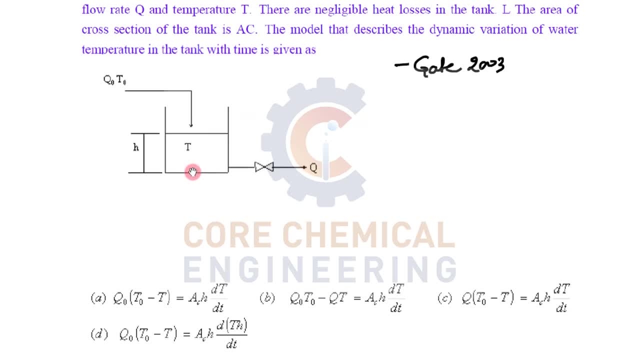 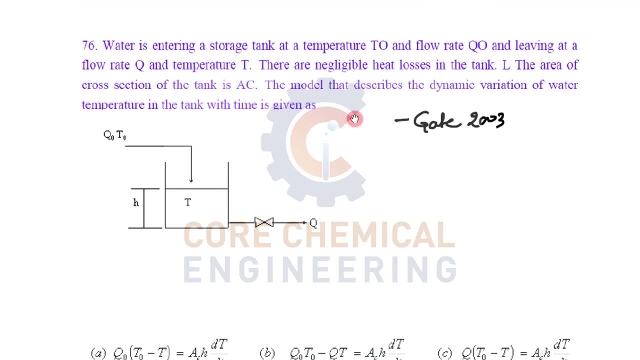 the area of cross section of the tank is ac, ac, not total ac. the model- the model describes the dynamic variations of water temperature in the tank with their time is given as so simplest. we have to do the energy when s for this tank, so we can. these are the options which has been given now we have